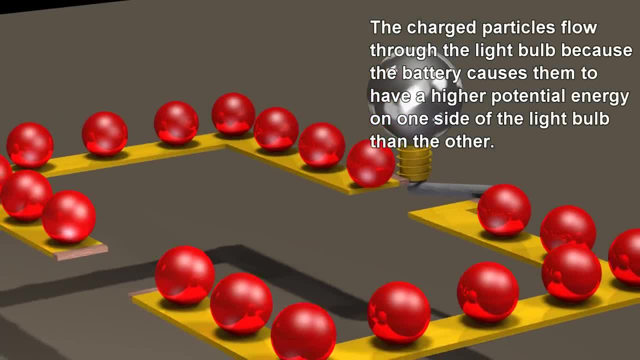 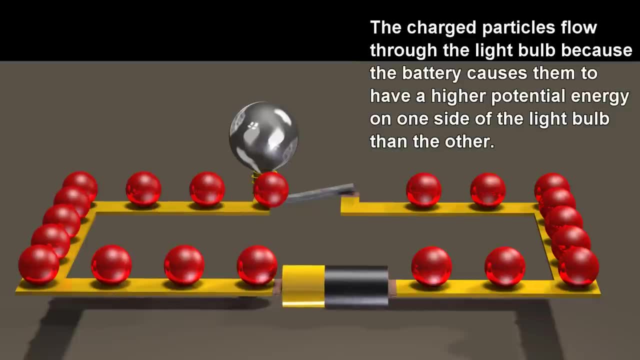 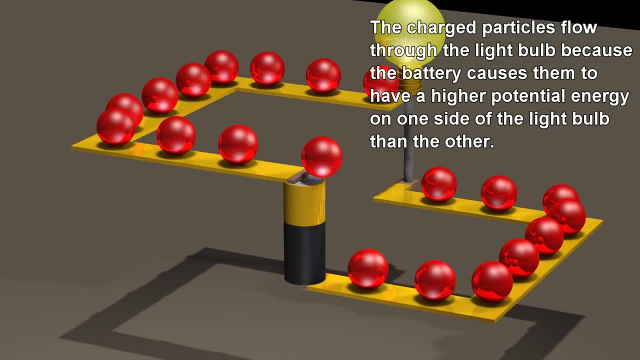 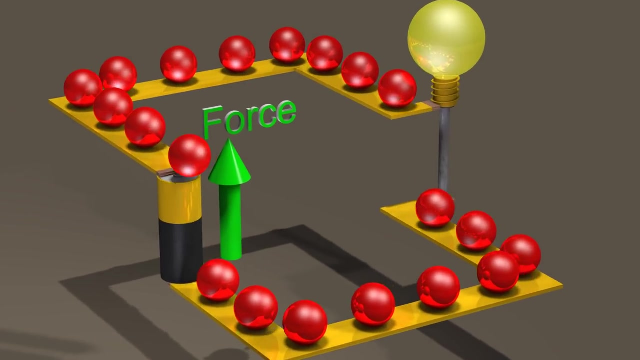 The charged particles flow through the light bulb because the battery causes them to have a higher potential energy on one side of the light bulb than the other. This potential energy is what we refer to as voltage. This potential energy is what we refer to as voltage. 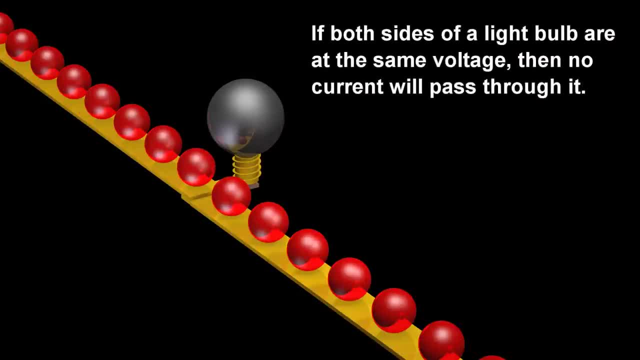 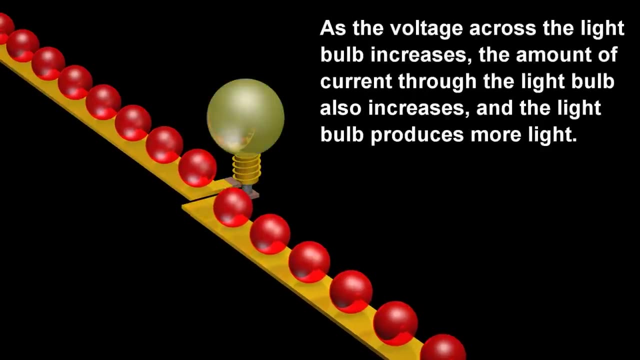 If both sides of a light bulb are at the same voltage, then no current will pass through it. As the voltage across the light bulb increases, the amount of current through the light bulb also increases. As the voltage across the light bulb increases, the amount of current through the light bulb also increases. 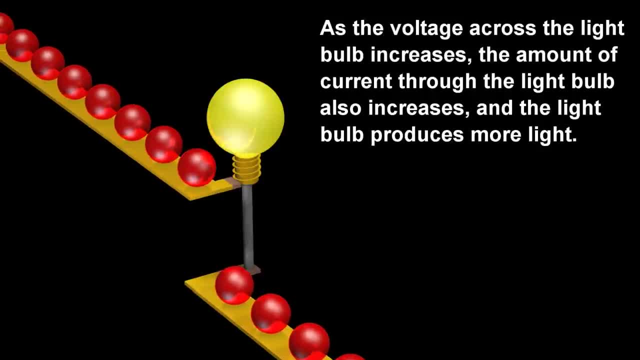 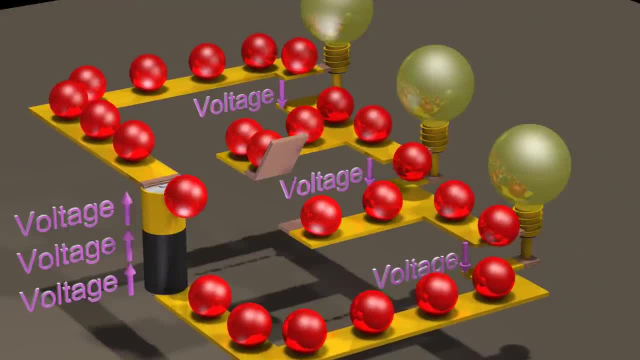 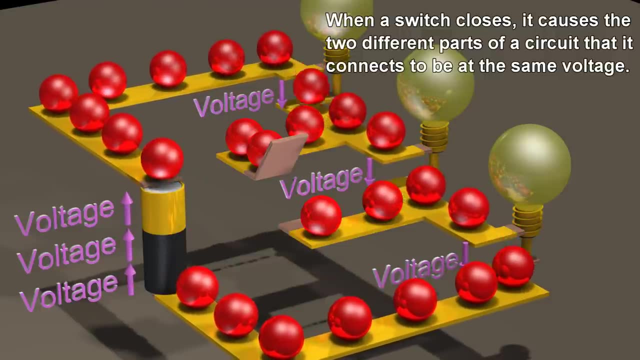 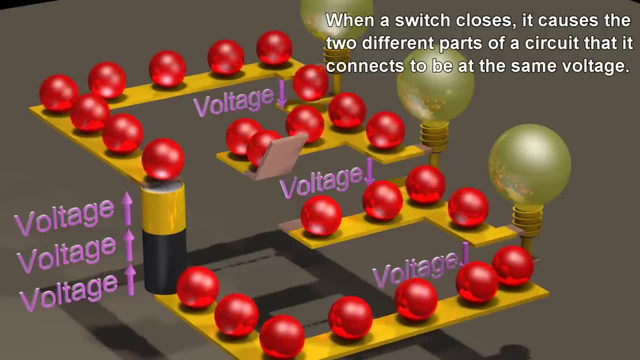 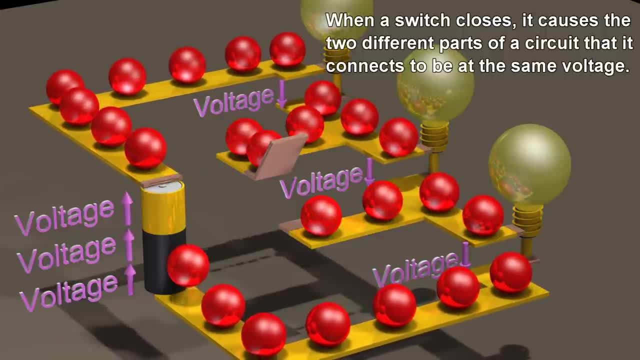 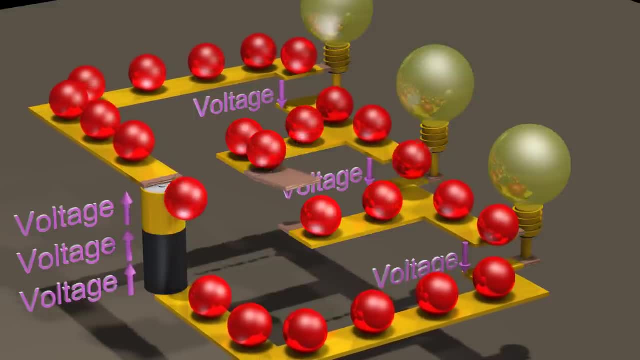 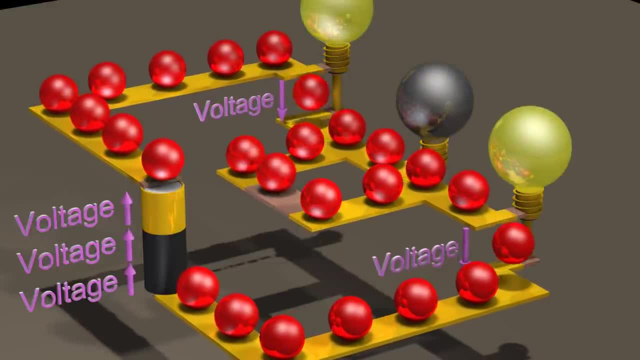 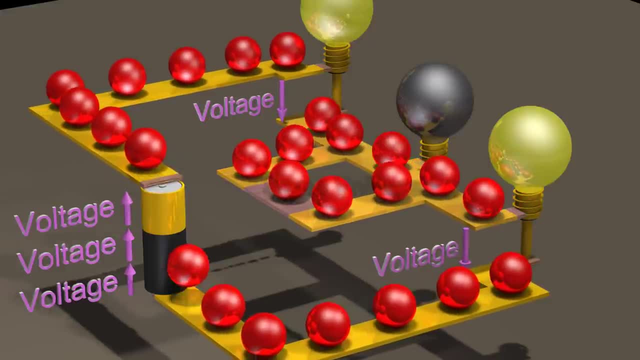 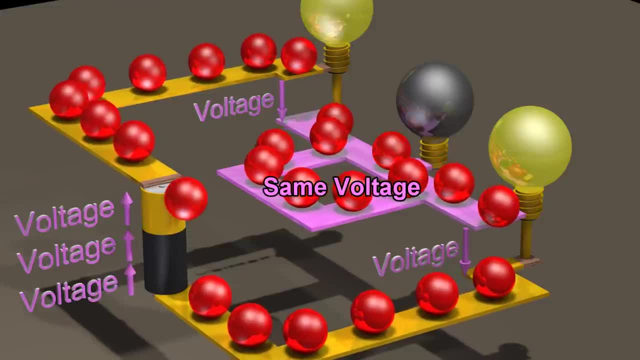 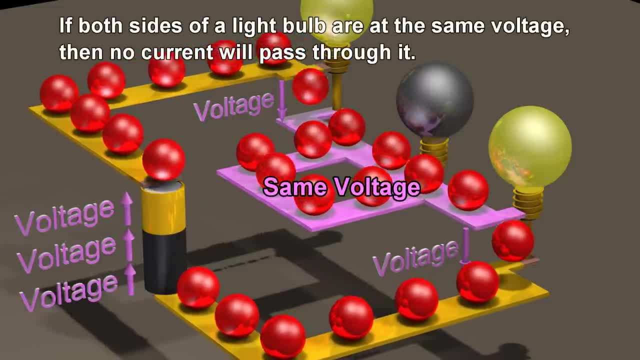 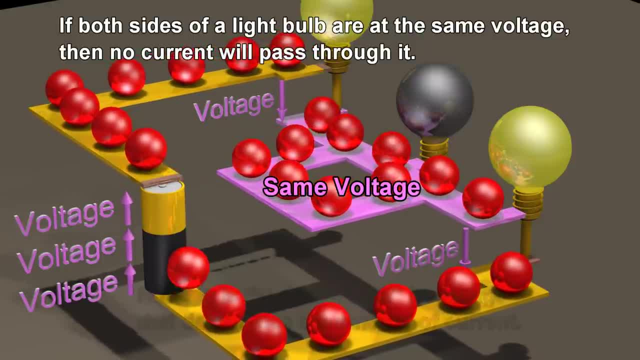 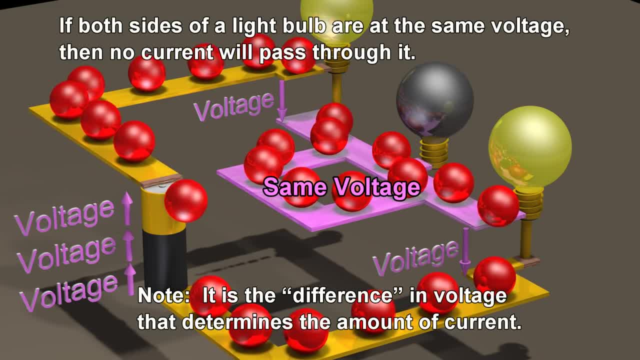 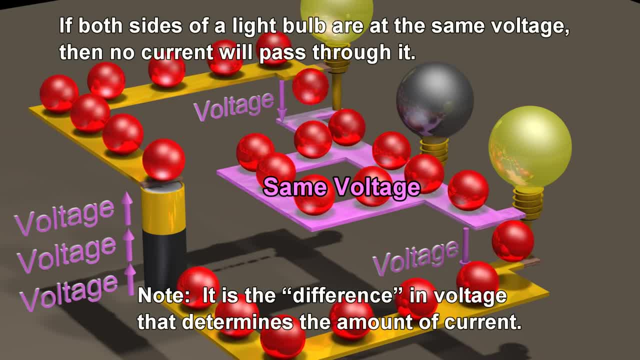 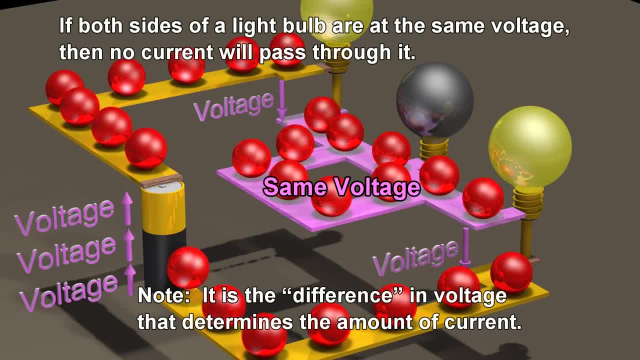 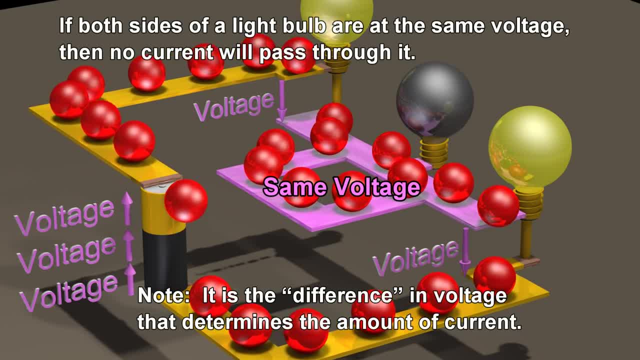 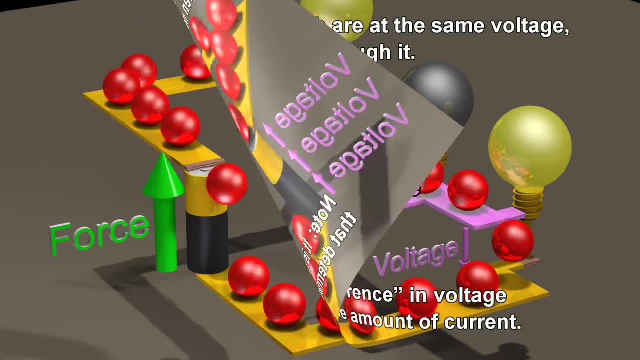 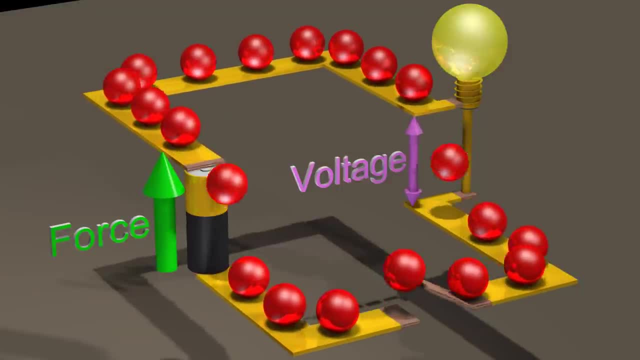 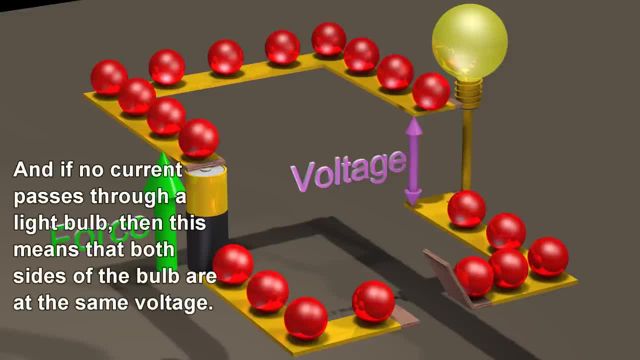 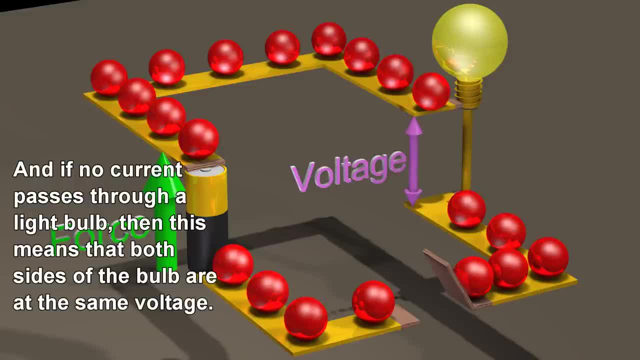 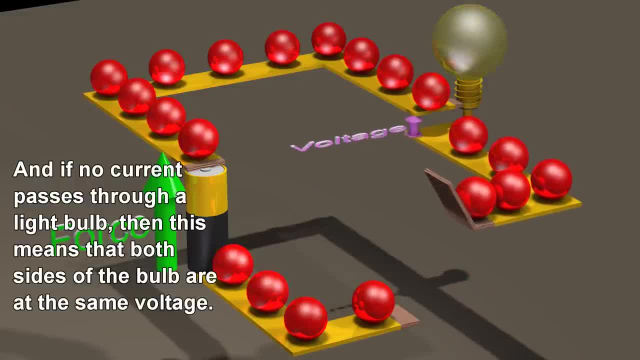 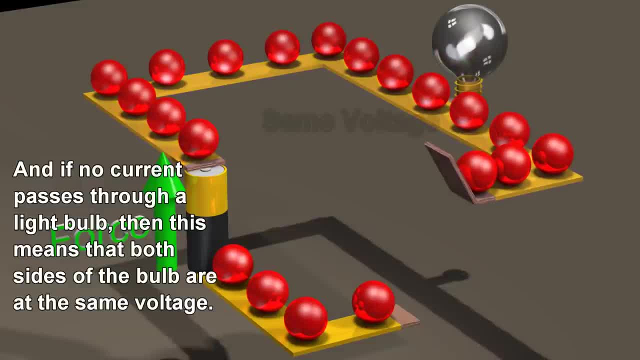 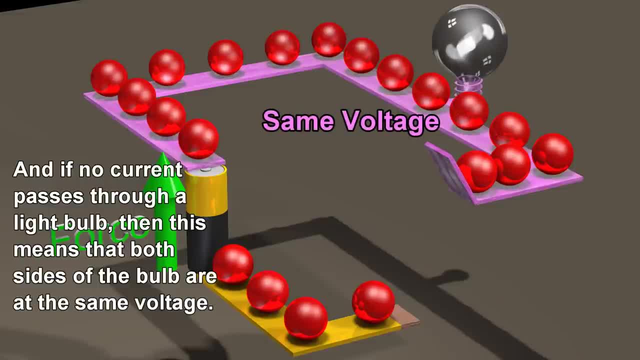 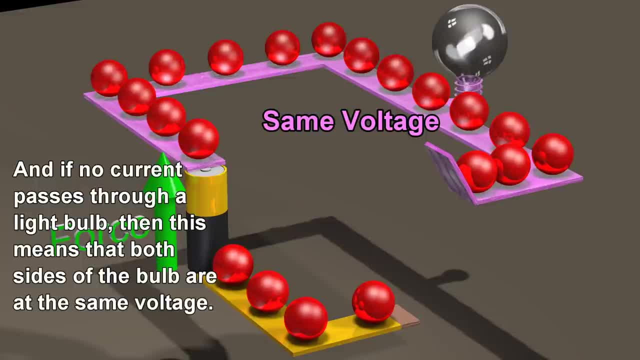 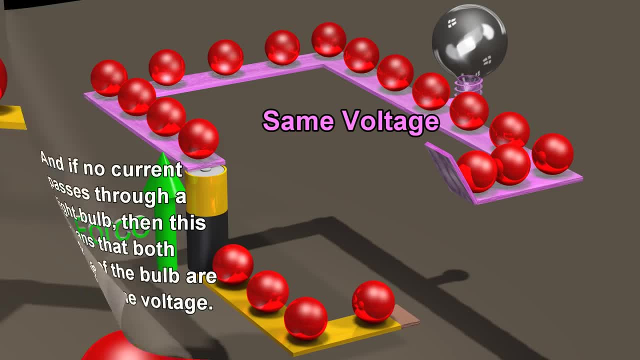 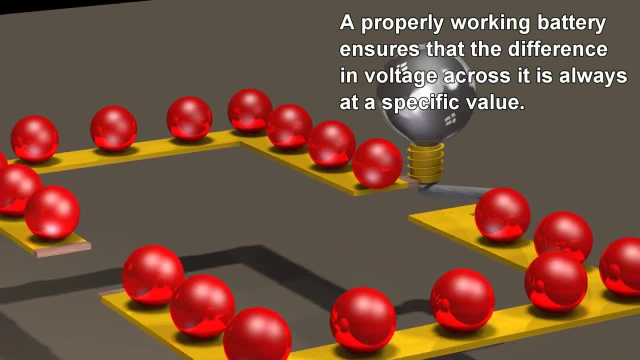 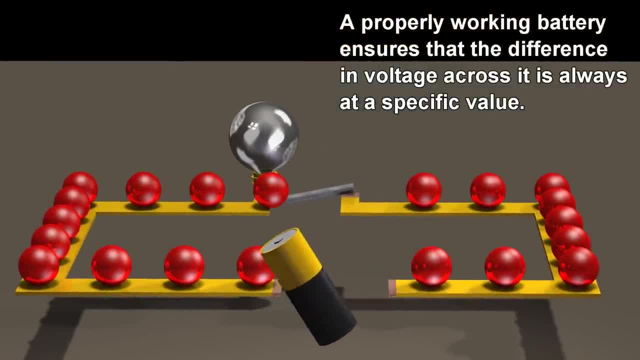 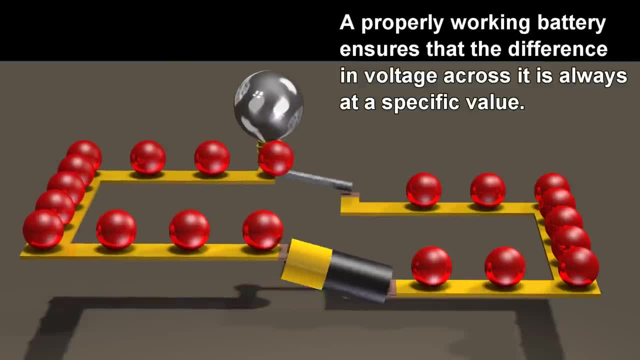 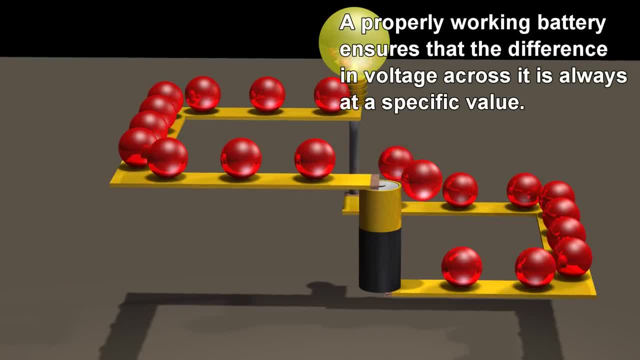 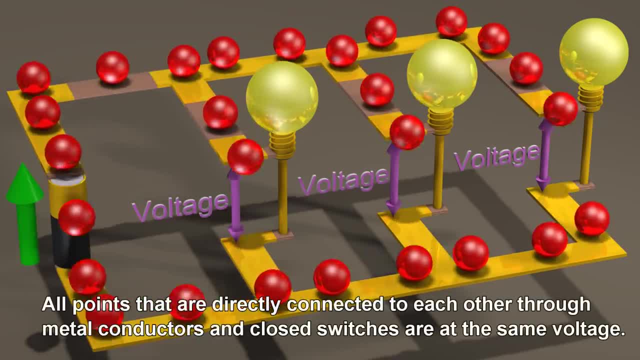 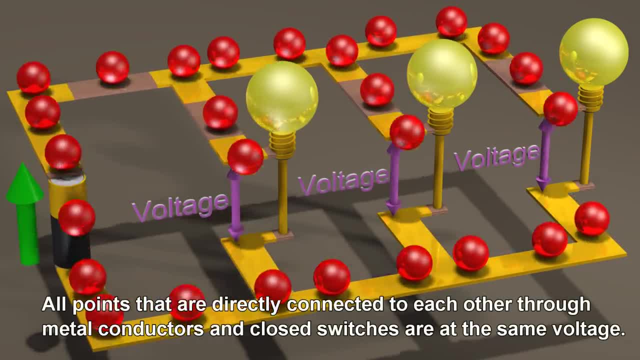 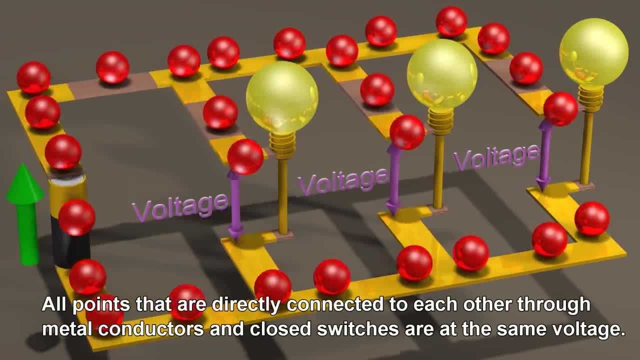 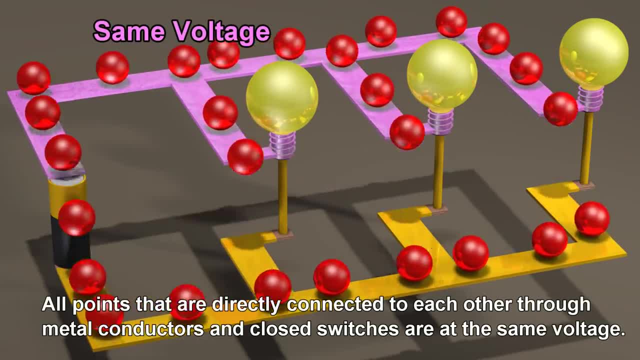 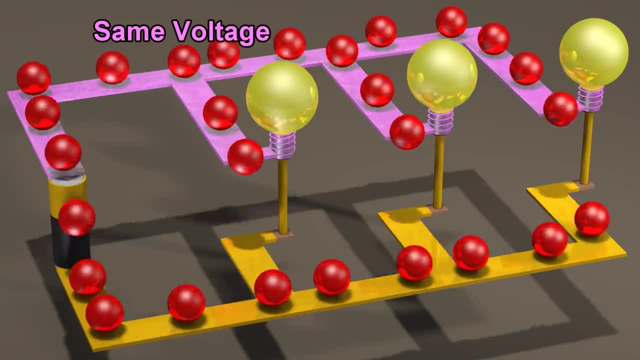 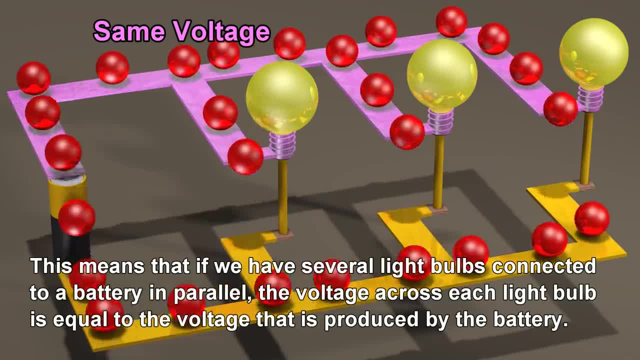 This means that if we have several light bulbs connected to a battery in parallel, the voltage across each light bulb is equal to the voltage that is produced by the battery. This means that if we have several light bulbs connected to a battery in parallel, the voltage across each light bulb is equal to the voltage that is produced by the battery. 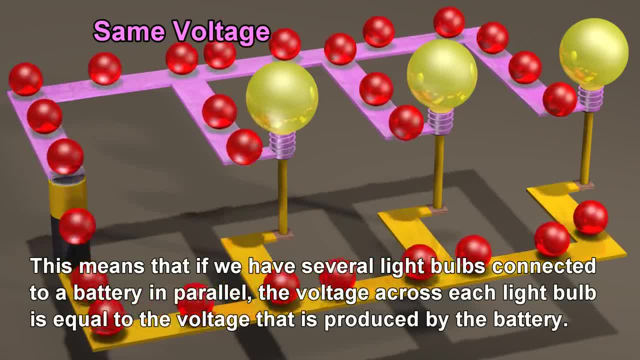 This means that if we have several light bulbs connected to a battery in parallel, the voltage across each light bulb is equal to the voltage that is produced by the battery. This means that if we have several light bulbs connected to a battery in parallel, the voltage across each light bulb is equal to the voltage that is produced by the battery. 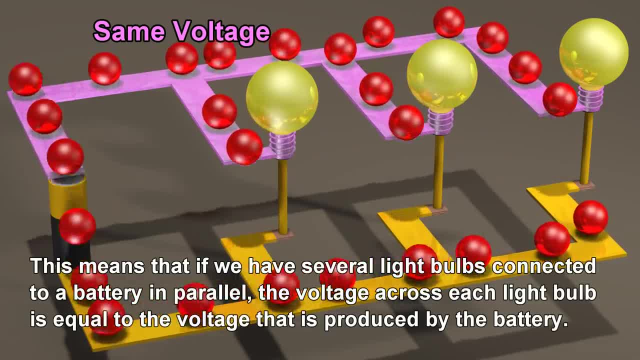 This means that if we have several light bulbs connected to a battery in parallel, the voltage across each light bulb is equal to the voltage that is produced by the battery. This means that if we have several light bulbs connected to a battery in parallel, the voltage across each light bulb is equal to the voltage that is produced by the battery. 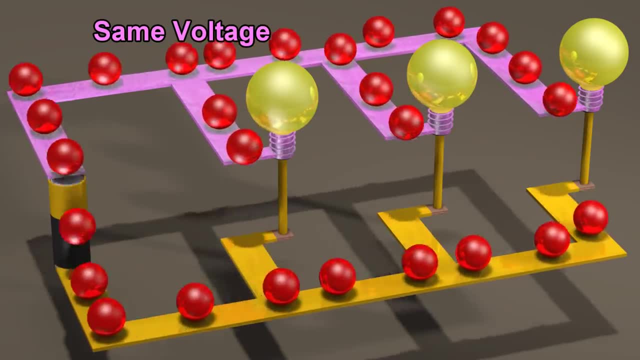 This means that if we have several light bulbs connected to a battery in parallel, the voltage across each light bulb is equal to the voltage that is produced by the battery. This means that if we have several light bulbs connected to a battery in parallel, the voltage across each light bulb is equal to the voltage that is produced by the battery. 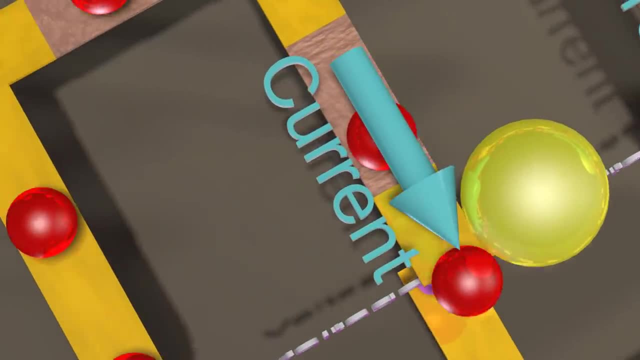 This means that if we have several light bulbs connected to a battery in parallel, the voltage across each light bulb is equal to the voltage that is produced by the battery. This means that if we have several light bulbs connected to a battery in parallel, the voltage across each light bulb is equal to the voltage that is produced by the battery. 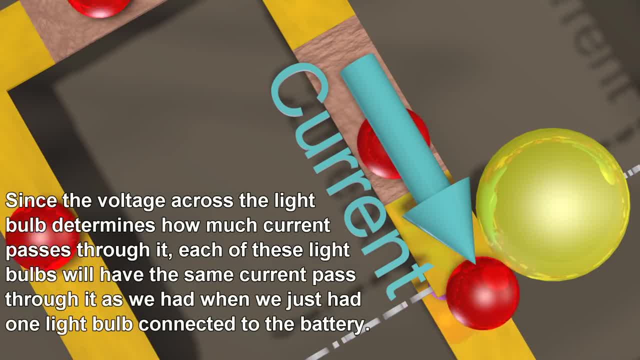 This means that if we have several light bulbs connected to a battery in parallel, the voltage across each light bulb is equal to the voltage that is produced by the battery. This means that if we have several light bulbs connected to a battery in parallel, the voltage across each light bulb is equal to the voltage that is produced by the battery. 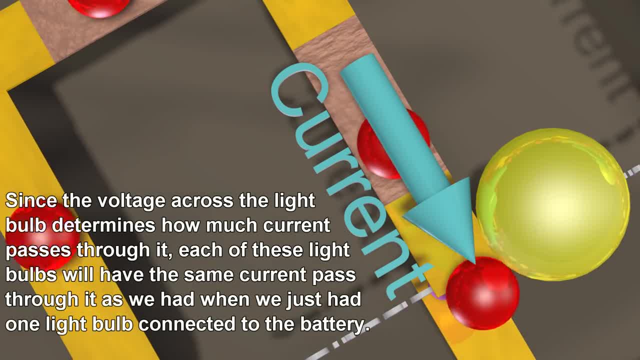 This means that if we have several light bulbs connected to a battery in parallel, the voltage across each light bulb is equal to the voltage that is produced by the battery. This means that if we have several light bulbs connected to a battery in parallel, the voltage across each light bulb is equal to the voltage that is produced by the battery. 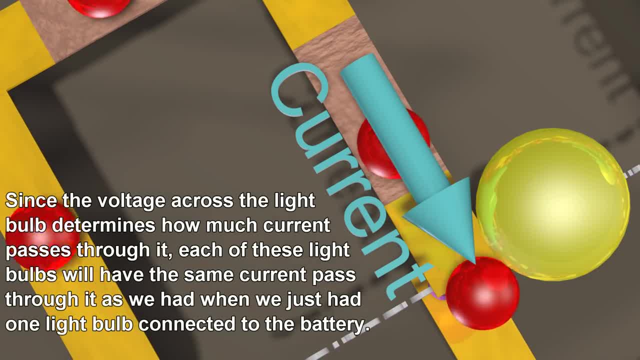 This means that if we have several light bulbs connected to a battery in parallel, the voltage across each light bulb is equal to the voltage that is produced by the battery. This means that if we have several light bulbs connected to a battery in parallel, the voltage across each light bulb is equal to the voltage that is produced by the battery. 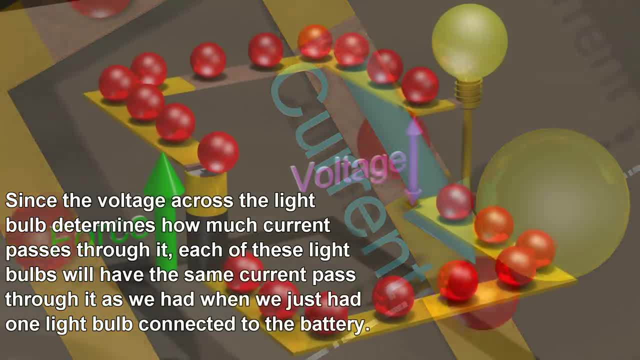 This means that if we have several light bulbs connected to a battery in parallel, the voltage across each light bulb is equal to the voltage that is produced by the battery. This means that if we have several light bulbs connected to a battery in parallel, the voltage across each light bulb is equal to the voltage that is produced by the battery. 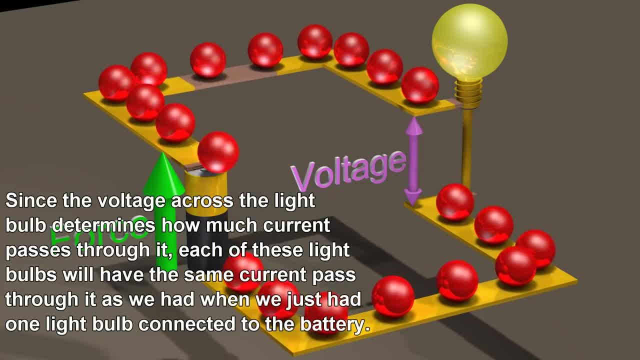 This means that if we have several light bulbs connected to a battery in parallel, the voltage across each light bulb is equal to the voltage that is produced by the battery. This means that if we have several light bulbs connected to a battery in parallel, the voltage across each light bulb is equal to the voltage that is produced by the battery. 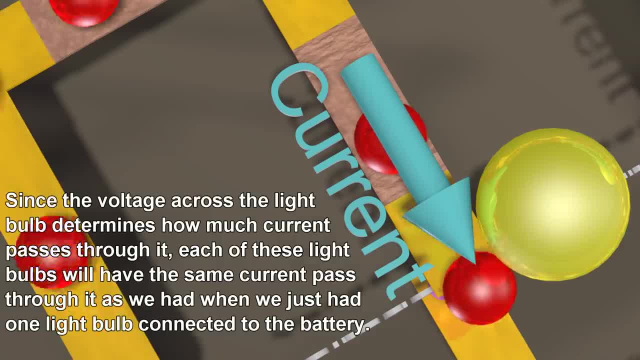 This means that if we have several light bulbs connected to a battery in parallel, the voltage across each light bulb is equal to the voltage that is produced by the battery. This means that if we have several light bulbs connected to a battery in parallel, the voltage across each light bulb is equal to the voltage that is produced by the battery. 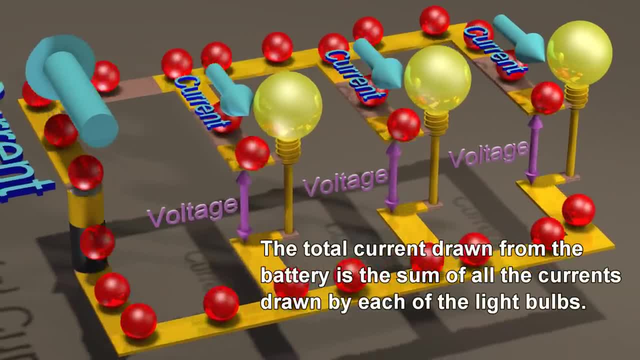 This means that if we have several light bulbs connected to a battery in parallel, the voltage across each light bulb is equal to the voltage that is produced by the battery. This means that if we have several light bulbs connected to a battery in parallel, the voltage across each light bulb is equal to the voltage that is produced by the battery. 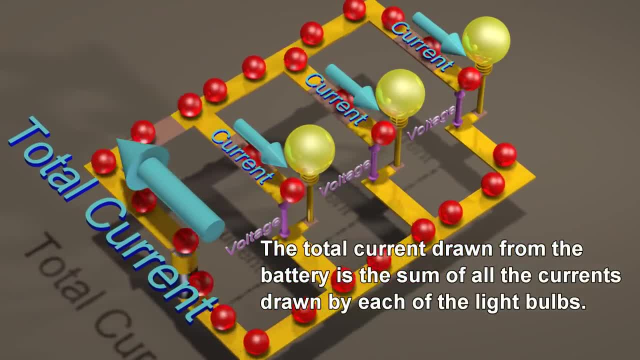 This means that if we have several light bulbs connected to a battery in parallel, the voltage across each light bulb is equal to the voltage that is produced by the battery. This means that if we have several light bulbs connected to a battery in parallel, the voltage across each light bulb is equal to the voltage that is produced by the battery. 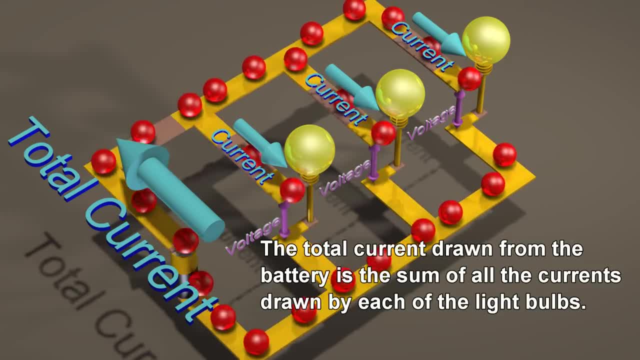 This means that if we have several light bulbs connected to a battery in parallel, the voltage across each light bulb is equal to the voltage that is produced by the battery. This means that if we have several light bulbs connected to a battery in parallel, the voltage across each light bulb is equal to the voltage that is produced by the battery. 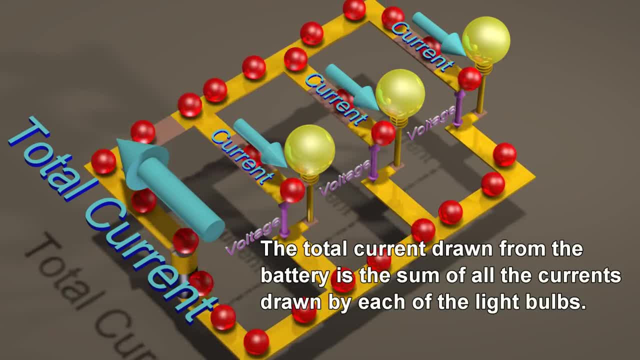 This means that if we have several light bulbs connected to a battery in parallel, the voltage across each light bulb is equal to the voltage that is produced by the battery. This means that if we have several light bulbs connected to a battery in parallel, the voltage across each light bulb is equal to the voltage that is produced by the battery. 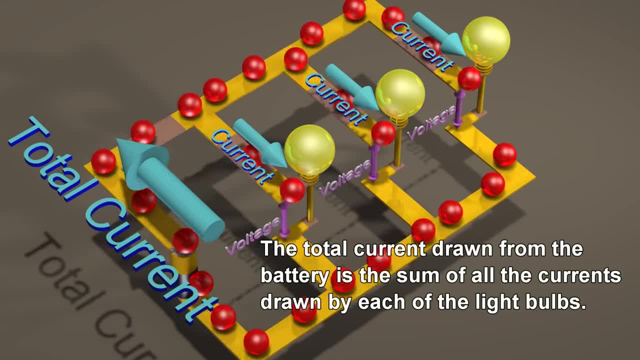 This means that if we have several light bulbs connected to a battery in parallel, the voltage across each light bulb is equal to the voltage that is produced by the battery. This means that if we have several light bulbs connected to a battery in parallel, the voltage across each light bulb is equal to the voltage that is produced by the battery. 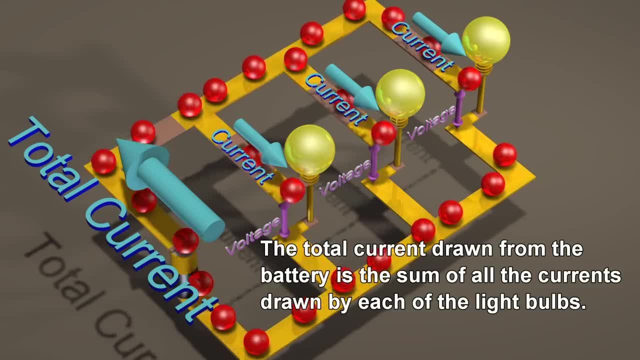 This means that if we have several light bulbs connected to a battery in parallel, the voltage across each light bulb is equal to the voltage that is produced by the battery. This means that if we have several light bulbs connected to a battery in parallel, the voltage across each light bulb is equal to the voltage that is produced by the battery. 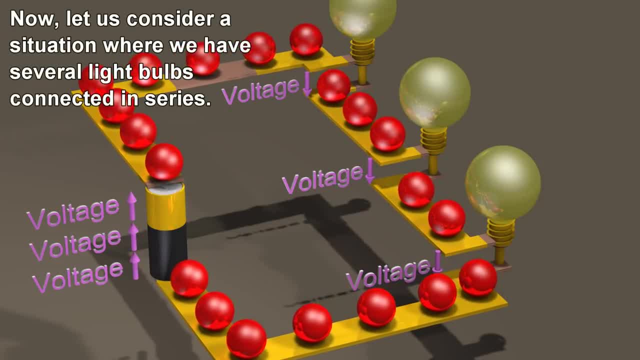 This means that if we have several light bulbs connected to a battery in parallel, the voltage across each light bulb is equal to the voltage that is produced by the battery. This means that if we have several light bulbs connected to a battery in parallel, the voltage across each light bulb is equal to the voltage that is produced by the battery. 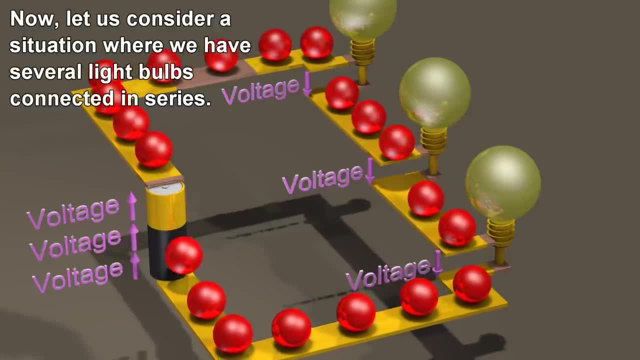 This means that if we have several light bulbs connected to a battery in parallel, the voltage across each light bulb is equal to the voltage that is produced by the battery. This means that if we have several light bulbs connected to a battery in parallel, the voltage across each light bulb is equal to the voltage that is produced by the battery. 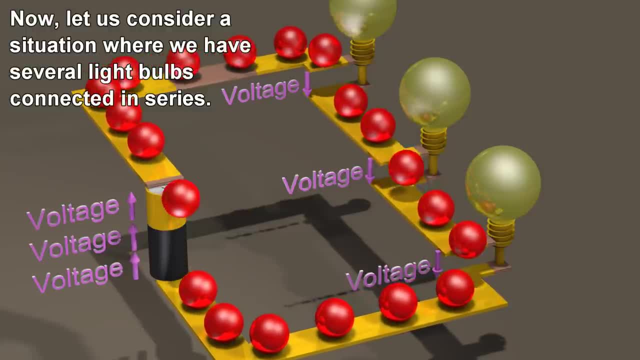 This means that if we have several light bulbs connected to a battery in parallel, the voltage across each light bulb is equal to the voltage that is produced by the battery. This means that if we have several light bulbs connected to a battery in parallel, the voltage across each light bulb is equal to the voltage that is produced by the battery. 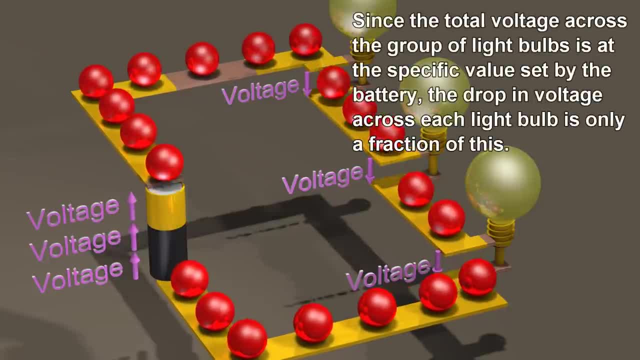 This means that if we have several light bulbs connected to a battery in parallel, the voltage across each light bulb is equal to the voltage that is produced by the battery. This means that if we have several light bulbs connected to a battery in parallel, the voltage across each light bulb is equal to the voltage that is produced by the battery. 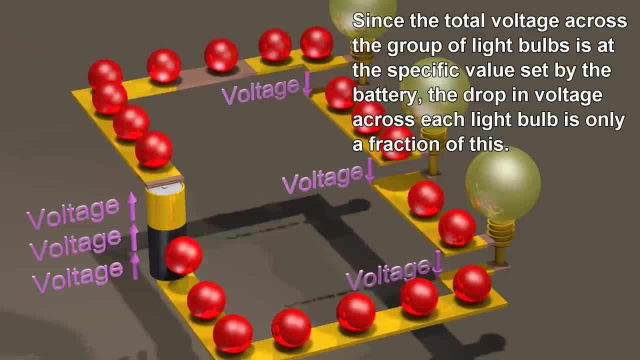 This means that if we have several light bulbs connected to a battery in parallel, the voltage across each light bulb is equal to the voltage that is produced by the battery. This means that if we have several light bulbs connected to a battery in parallel, the voltage across each light bulb is equal to the voltage that is produced by the battery. 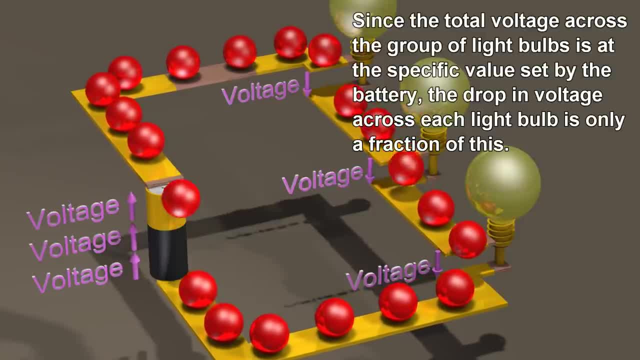 This means that if we have several light bulbs connected to a battery in parallel, the voltage across each light bulb is equal to the voltage that is produced by the battery. This means that if we have several light bulbs connected to a battery in parallel, the voltage across each light bulb is equal to the voltage that is produced by the battery. 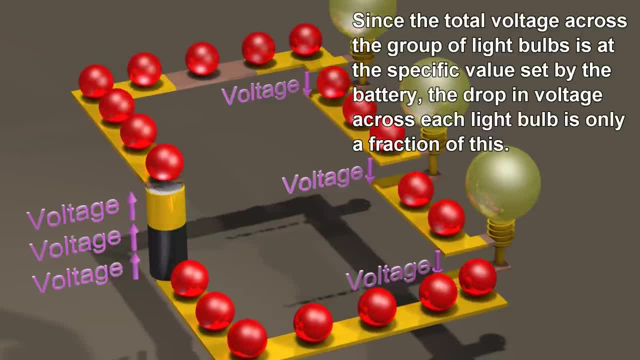 This means that if we have several light bulbs connected to a battery in parallel, the voltage across each light bulb is equal to the voltage that is produced by the battery. This means that if we have several light bulbs connected to a battery in parallel, the voltage across each light bulb is equal to the voltage that is produced by the battery. 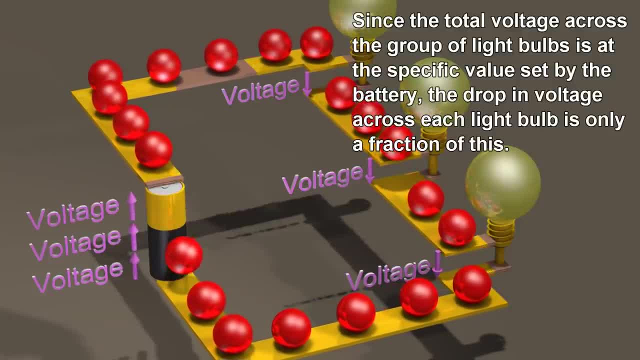 This means that if we have several light bulbs connected to a battery in parallel, the voltage across each light bulb is equal to the voltage that is produced by the battery. This means that if we have several light bulbs connected to a battery in parallel, the voltage across each light bulb is equal to the voltage that is produced by the battery. 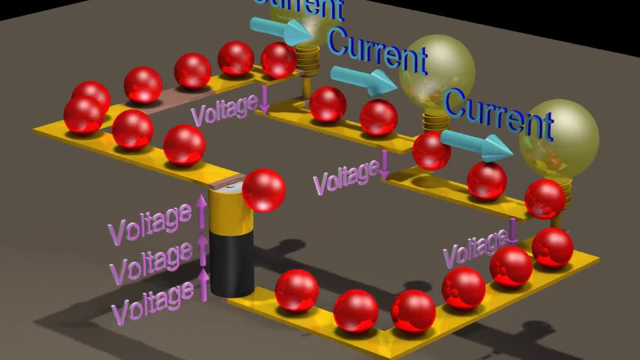 This means that if we have several light bulbs connected to a battery in parallel, the voltage across each light bulb is equal to the voltage that is produced by the battery. This means that if we have several light bulbs connected to a battery in parallel, the voltage across each light bulb is equal to the voltage that is produced by the battery. 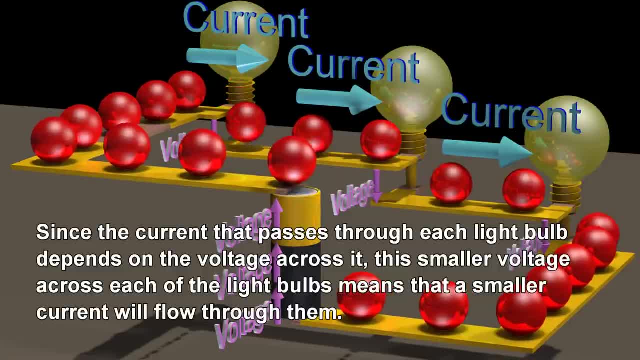 This means that if we have several light bulbs connected to a battery in parallel, the voltage across each light bulb is equal to the voltage that is produced by the battery. This means that if we have several light bulbs connected to a battery in parallel, the voltage across each light bulb is equal to the voltage that is produced by the battery. 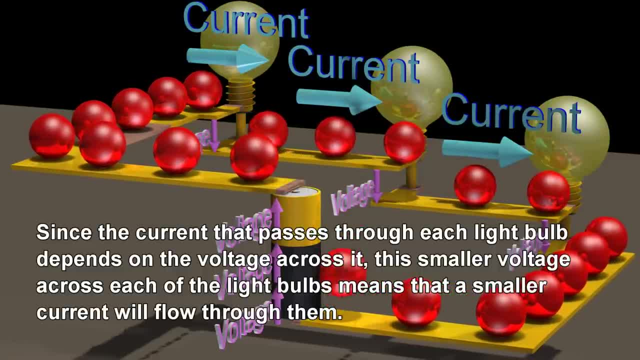 This means that if we have several light bulbs connected to a battery in parallel, the voltage across each light bulb is equal to the voltage that is produced by the battery. This means that if we have several light bulbs connected to a battery in parallel, the voltage across each light bulb is equal to the voltage that is produced by the battery. 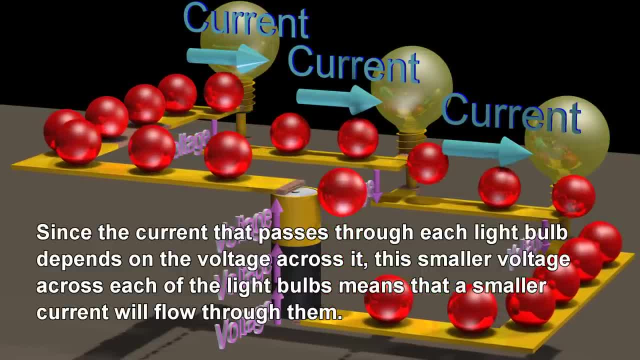 This means that if we have several light bulbs connected to a battery in parallel, the voltage across each light bulb is equal to the voltage that is produced by the battery. This means that if we have several light bulbs connected to a battery in parallel, the voltage across each light bulb is equal to the voltage that is produced by the battery. 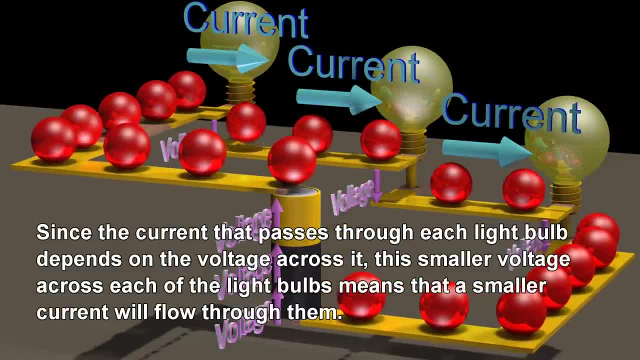 This means that if we have several light bulbs connected to a battery in parallel, the voltage across each light bulb is equal to the voltage that is produced by the battery. This means that if we have several light bulbs connected to a battery in parallel, the voltage across each light bulb is equal to the voltage that is produced by the battery. 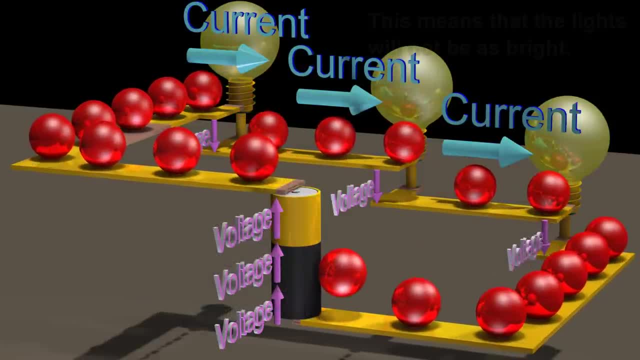 This means that if we have several light bulbs connected to a battery in parallel, the voltage across each light bulb is equal to the voltage that is produced by the battery. This means that if we have several light bulbs connected to a battery in parallel, the voltage across each light bulb is equal to the voltage that is produced by the battery. 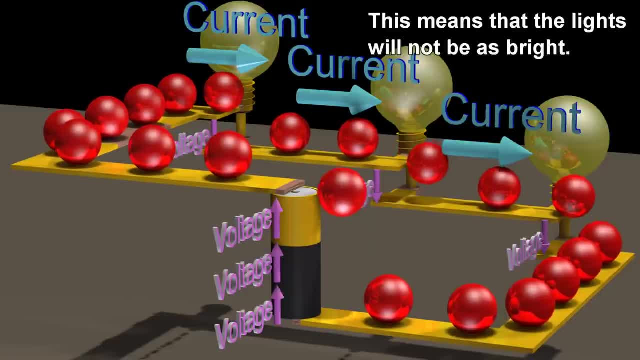 This means that if we have several light bulbs connected to a battery in parallel, the voltage across each light bulb is equal to the voltage that is produced by the battery. This means that if we have several light bulbs connected to a battery in parallel, the voltage across each light bulb is equal to the voltage that is produced by the battery. 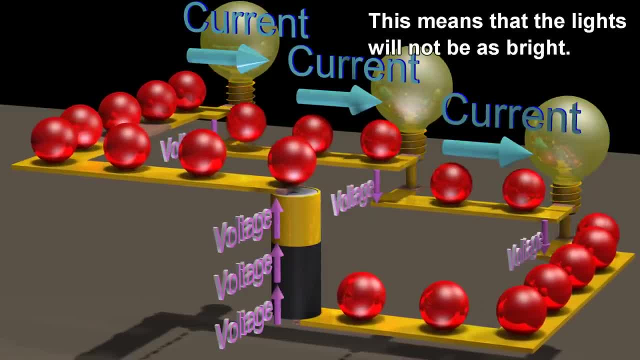 This means that if we have several light bulbs connected to a battery in parallel, the voltage across each light bulb is equal to the voltage that is produced by the battery. This means that if we have several light bulbs connected to a battery in parallel, the voltage across each light bulb is equal to the voltage that is produced by the battery. 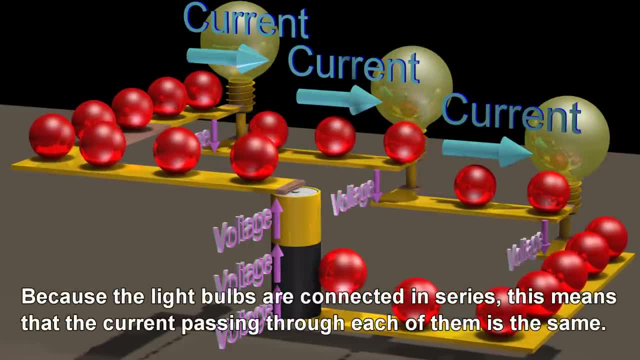 This means that if we have several light bulbs connected to a battery in parallel, the voltage across each light bulb is equal to the voltage that is produced by the battery. This means that if we have several light bulbs connected to a battery in parallel, the voltage across each light bulb is equal to the voltage that is produced by the battery. 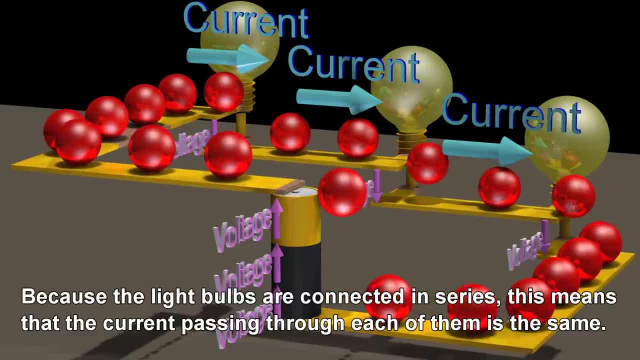 This means that if we have several light bulbs connected to a battery in parallel, the voltage across each light bulb is equal to the voltage that is produced by the battery. This means that if we have several light bulbs connected to a battery in parallel, the voltage across each light bulb is equal to the voltage that is produced by the battery. 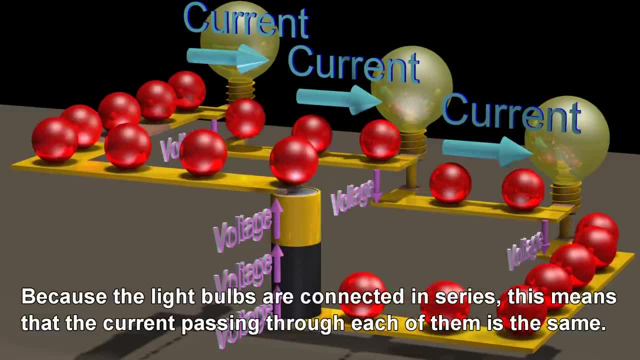 This means that if we have several light bulbs connected to a battery in parallel, the voltage across each light bulb is equal to the voltage that is produced by the battery. This means that if we have several light bulbs connected to a battery in parallel, the voltage across each light bulb is equal to the voltage that is produced by the battery. 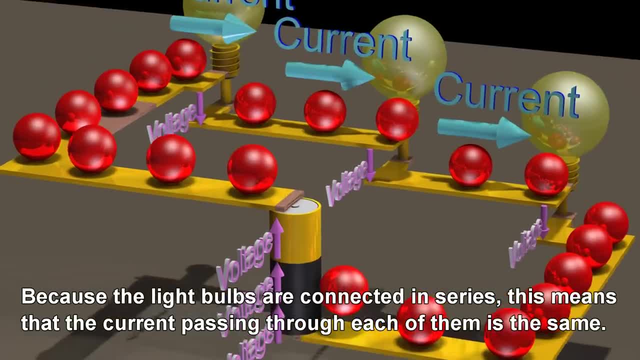 This means that if we have several light bulbs connected to a battery in parallel, the voltage across each light bulb is equal to the voltage that is produced by the battery. This means that if we have several light bulbs connected to a battery in parallel, the voltage across each light bulb is equal to the voltage that is produced by the battery. 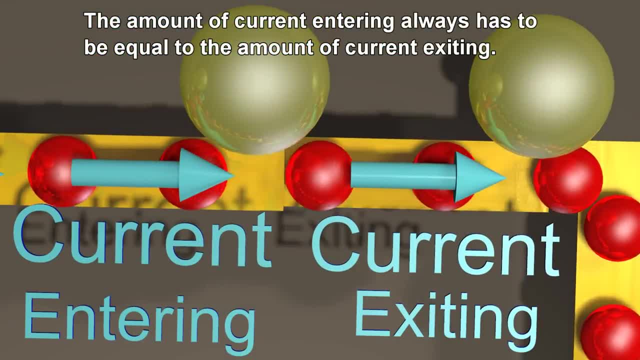 This means that if we have several light bulbs connected to a battery in parallel, the voltage across each light bulb is equal to the voltage that is produced by the battery. This means that if we have several light bulbs connected to a battery in parallel, the voltage across each light bulb is equal to the voltage that is produced by the battery. 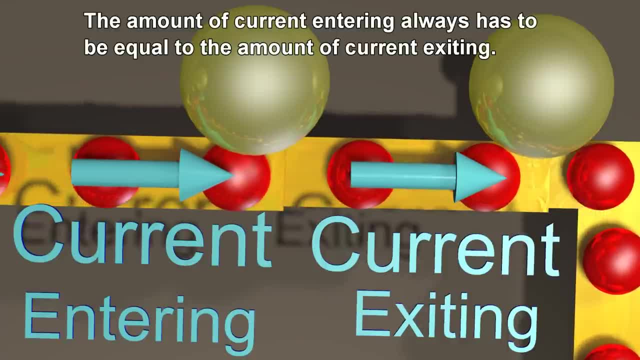 This means that if we have several light bulbs connected to a battery in parallel, the voltage across each light bulb is equal to the voltage that is produced by the battery. This means that if we have several light bulbs connected to a battery in parallel, the voltage across each light bulb is equal to the voltage that is produced by the battery. 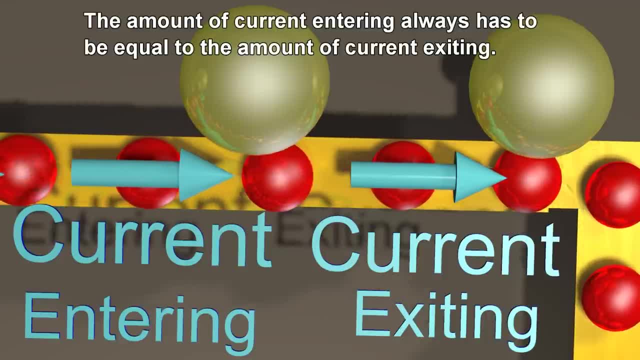 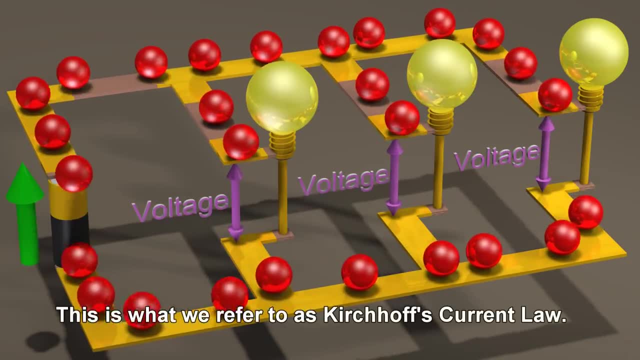 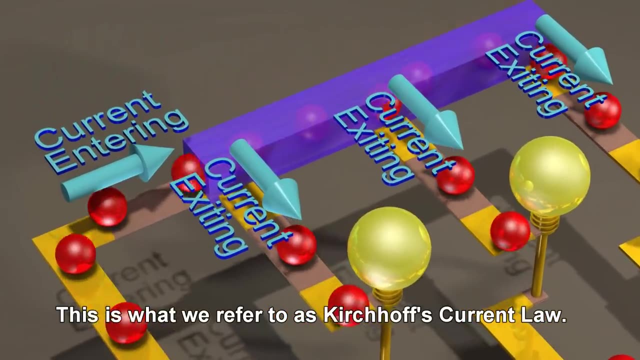 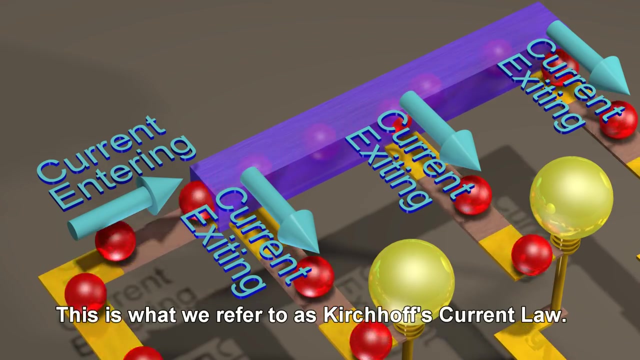 This means that if we have several light bulbs connected to a battery in parallel, the voltage across each light bulb is equal to the voltage that is produced by the battery. This is what we refer to as Kirchhoff's current law. This is what we refer to as Kirchhoff's current law.